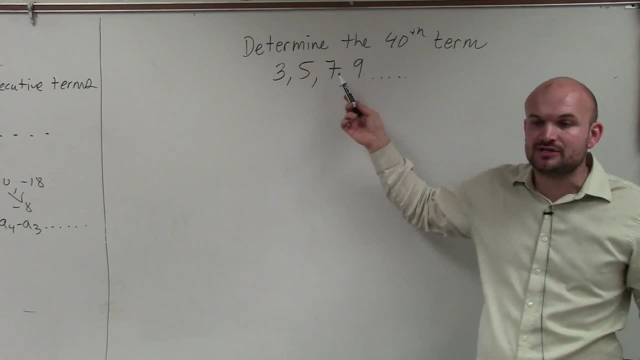 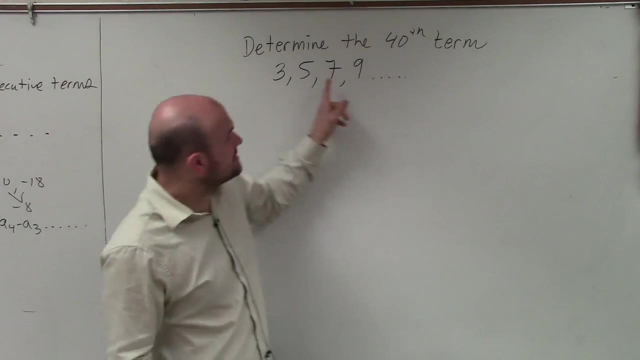 Yeah, you could subtract them, but this one's pretty obvious. You can see that the difference between your terms is 2.. Right, So to determine, you could easily just keep on adding 2 all the way up until you get to the 40th term. 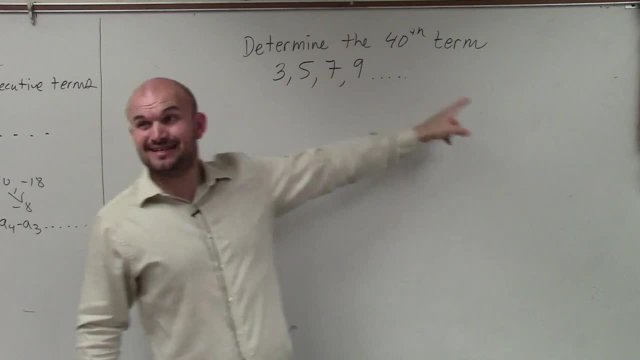 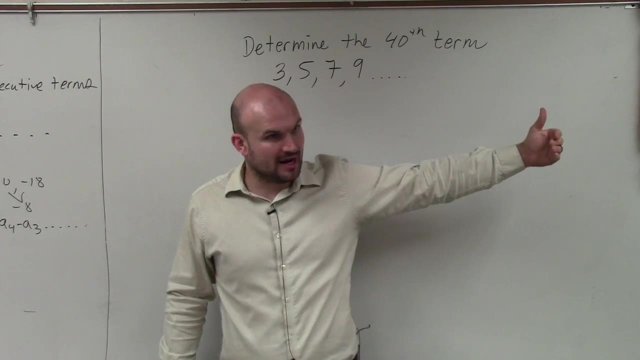 Right, That's the first term, second term, third term, fourth term, And you could keep on doing that to 40 terms. However, if you're taking a test, that's probably not the best use of your time, Right. 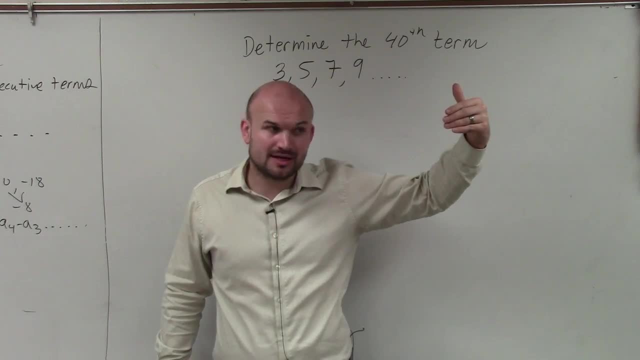 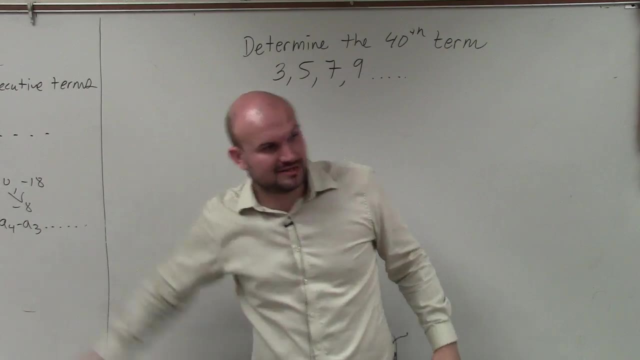 Or what if I gave you the 400th term? Are you really going to want to count all the terms adding 2 up to 400?? No, not really. So what we're going to want to use is our explicit formula, which I provided to you guys. 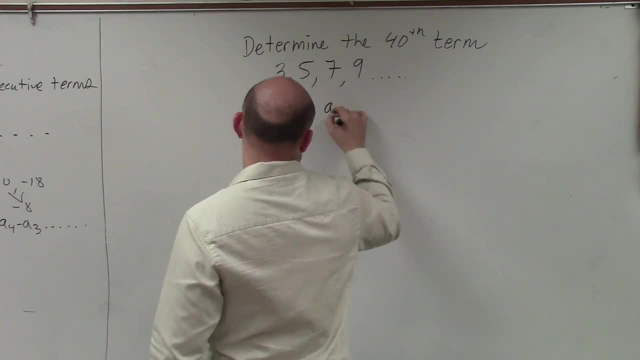 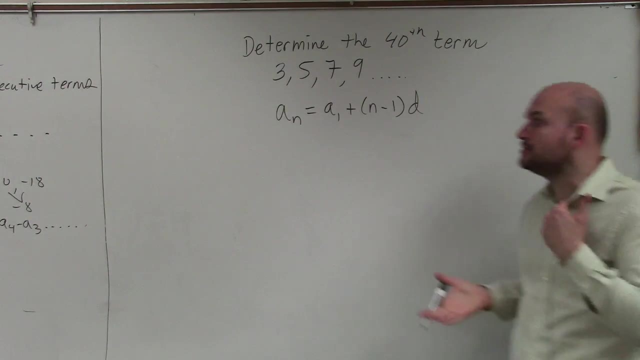 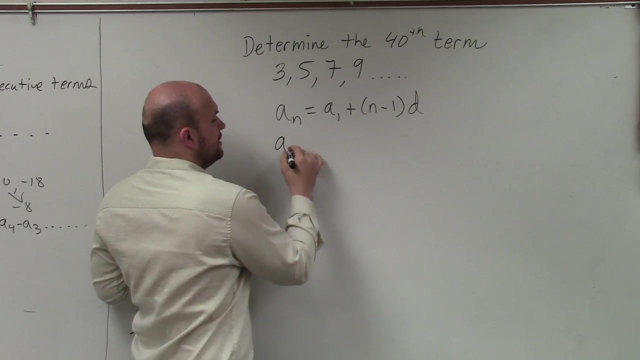 So the explicit formula is: a sub n equals a sub 1 plus n minus 1 times d. So now what we want to do is we need to determine what is the 40th term. So, just like we did last class period when we want to find, remember when we said: find the first term. 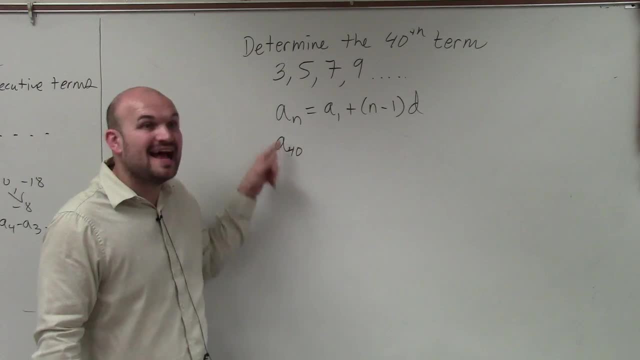 We plugged in 1 in for here, in for the a of a sub 1, and then that 1 got plugged in for the n- Do you guys remember that? And then we found the first number And then we did a sub 2.. 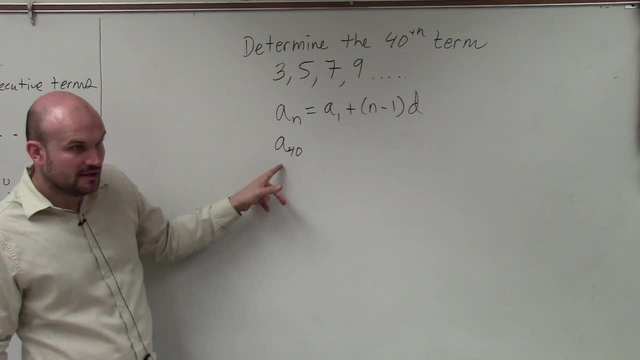 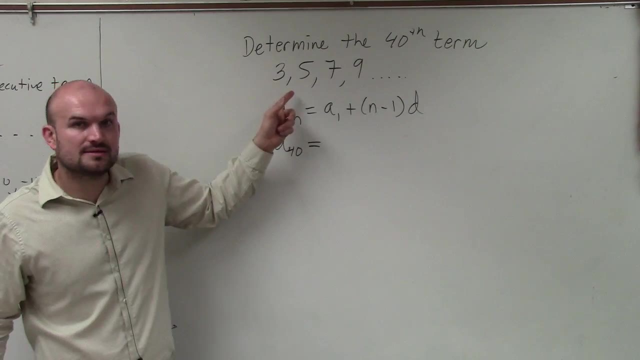 We plugged in 2.. We plugged in 2 in for n. So when we want to find a sub 40, we're going to plug 40 in for n. Then do we know what the first term in the sequence is? 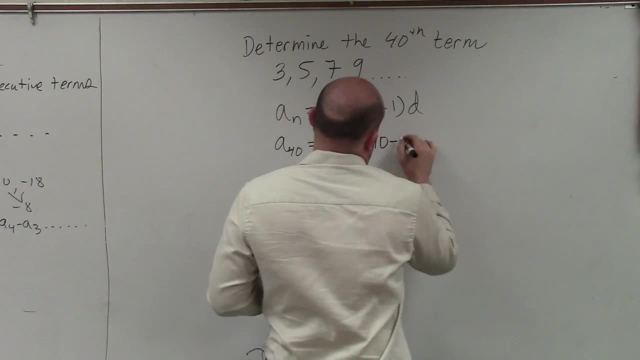 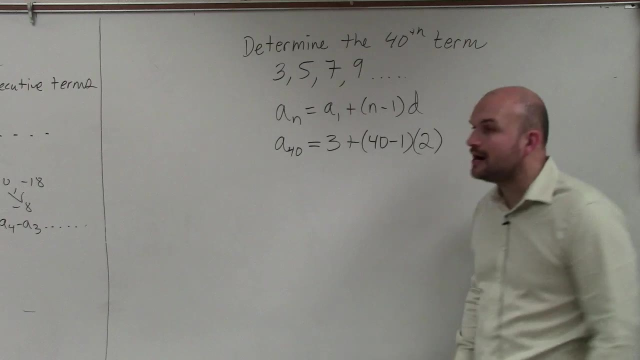 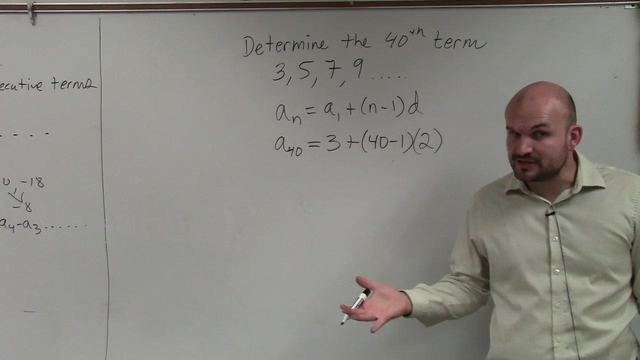 3. And then d is the difference, which is 2.. So now to find the 40th term. ladies and gentlemen, we have all the information we need. We just now need to simplify. Now make sure we apply. order of operations. 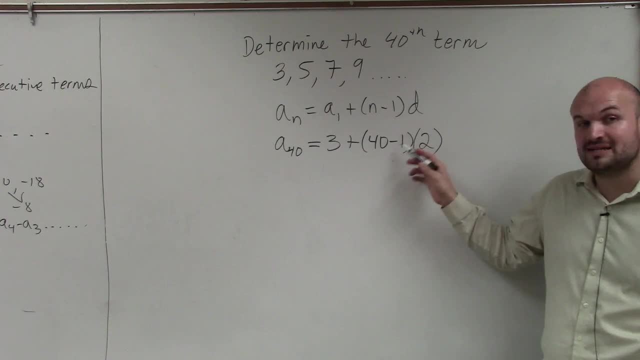 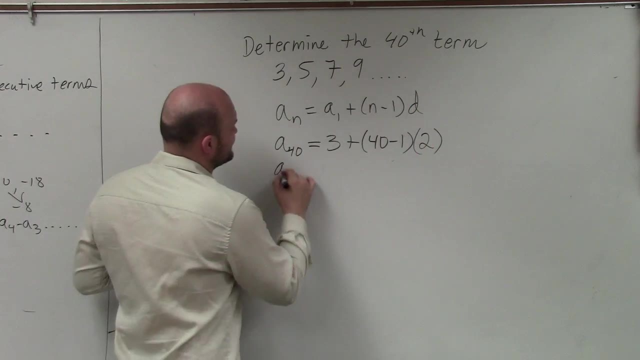 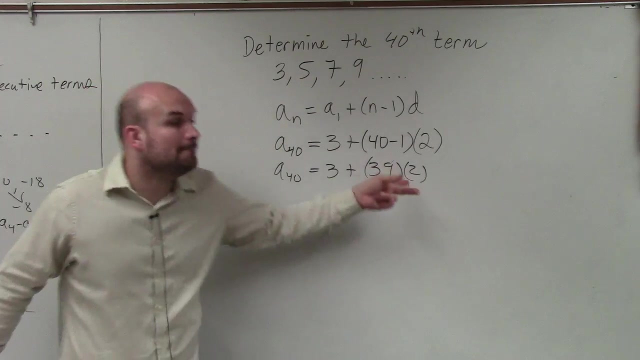 This is where a lot of students make mistakes. 40, you've got to do inside the parentheses first. 40 minus 1 is going to be 39. I'll just do this step by step. Then we have to make sure we multiply before we add. 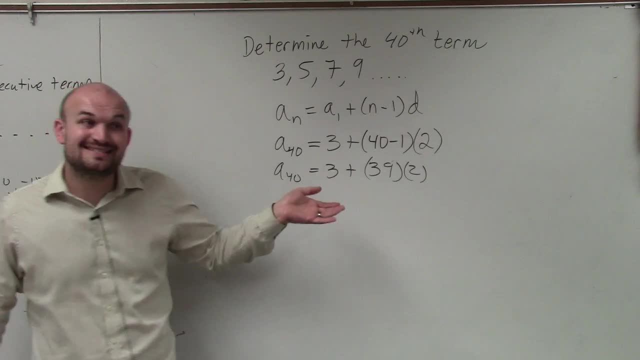 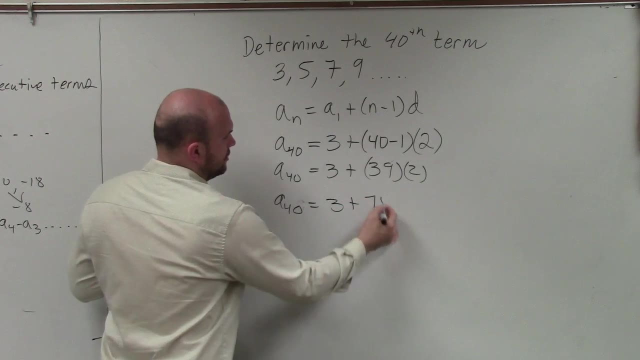 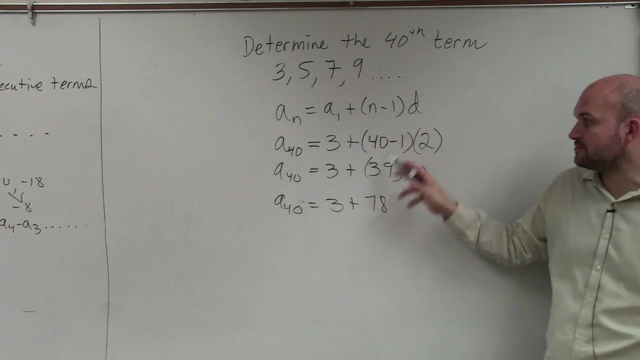 So 38,, 39,- sorry times- 2 is going to be 78.. Back up, What do you mean? like my work, Like from here to here. So all I did was I subtracted 40 minus 1 was 39..